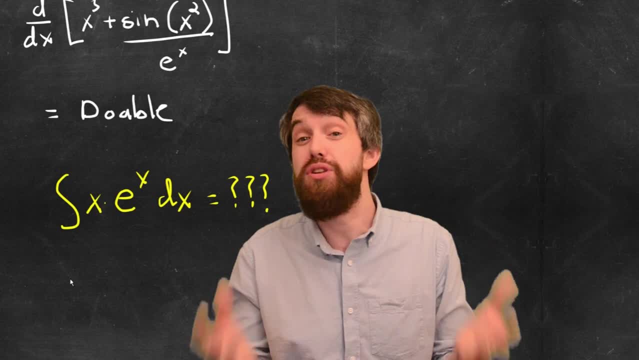 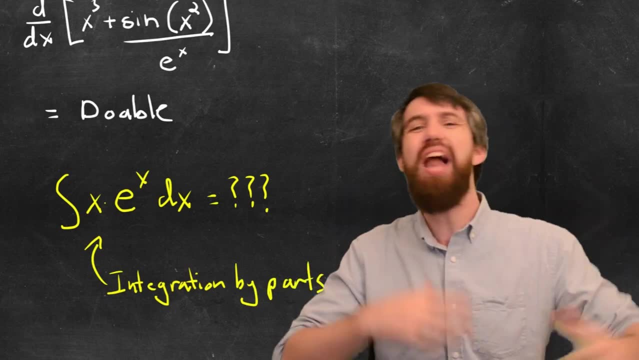 the amount of integrals that we're actually able to do. We're going to see, for example, that this x e to the x one can be done by a method called integration by parts. It sort of undoes the product rule, in the same way that u-substitution undid the chain rule. We'll see how to integrate. 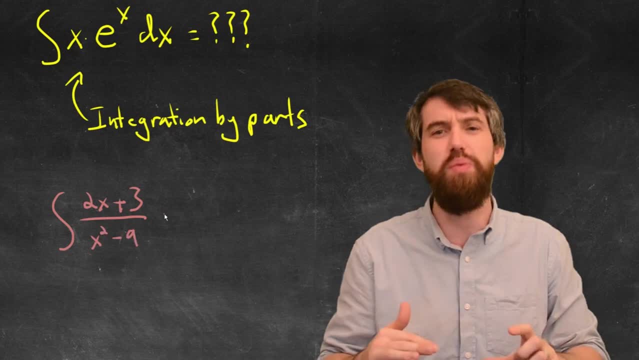 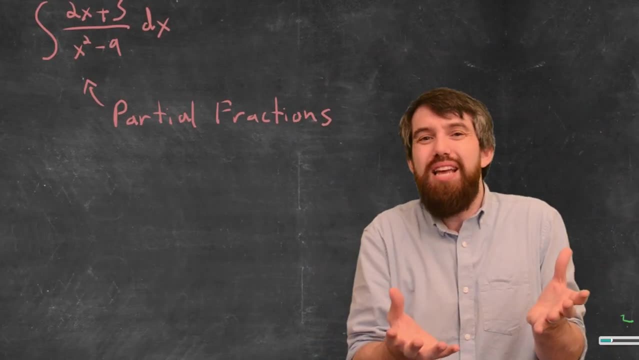 things that are rational functions: a polynomial on the top divided by a polynomial on the bottom. We're going to have a little bit of algebraic trickery called partial fractions. We're going to see how to integrate integrals that have a whole bunch of trigonometric terms. 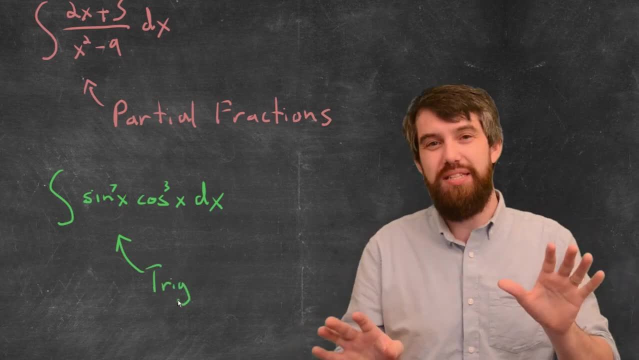 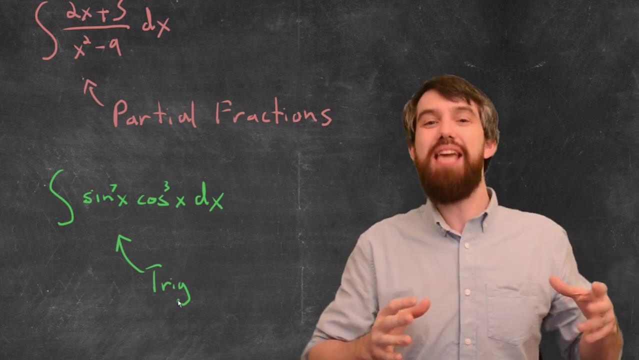 sines and cosines and so on. We're going to learn a whole bunch of these different integration methods, But what I like about integration is that, unlike differentiation integration, it isn't the case that we have an algebraic method for every type of integral. In fact, there's all kinds of integrals that you and 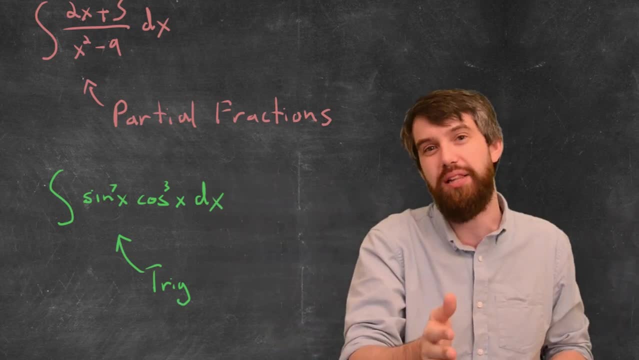 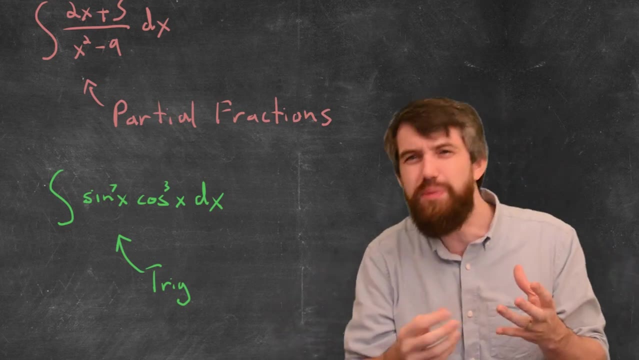 me and nobody else actually knows how to do, at least not algebraically. And indeed often when you're faced with an interesting integral, it's a little bit of sort of a crazy knot. You don't know what to do. You're supposed to make a substitution and you try to try. 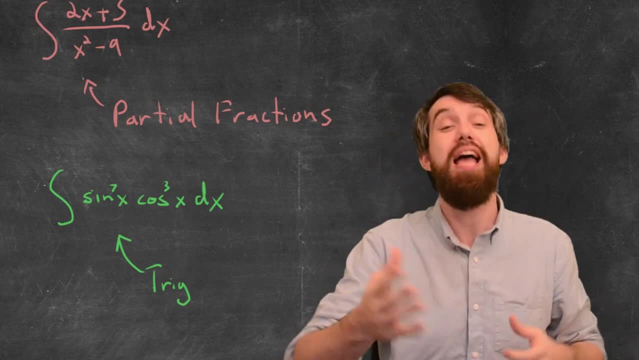 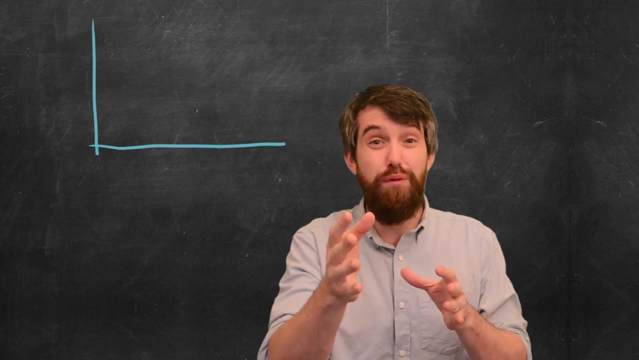 some method. You sort of pick away at it until you get a creative idea and then you're able to evaluate this integral. Sometimes you can do that, sometimes you can't. Now it gets a little bit interesting. We've seen before that the integral from a to b. 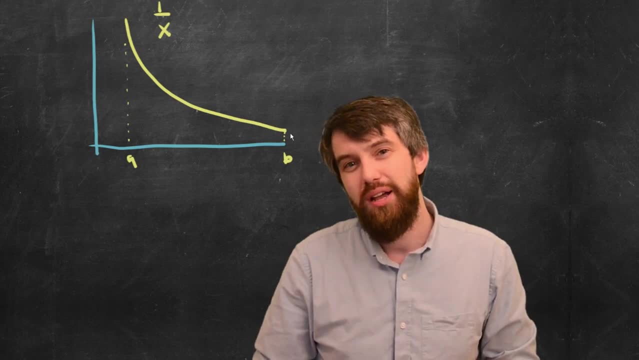 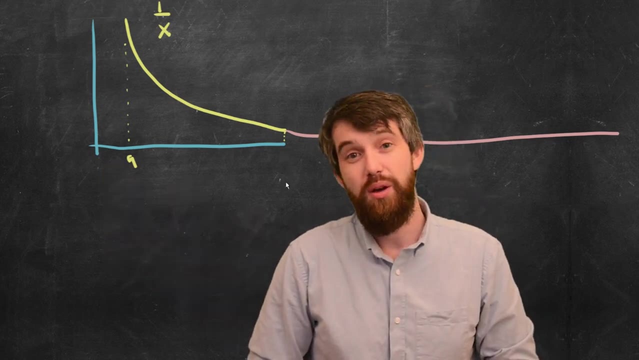 was just the same thing as the area under a curve. But what if b was infinity? What if this was the area under the curve from some spot all the way off to infinity? Well, it turns out that you can do these integrals and that they can sometimes actually be finite. 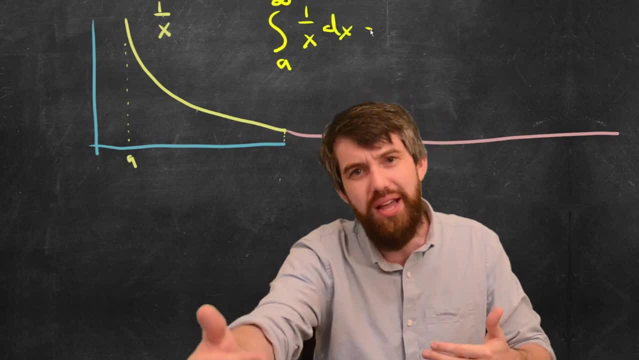 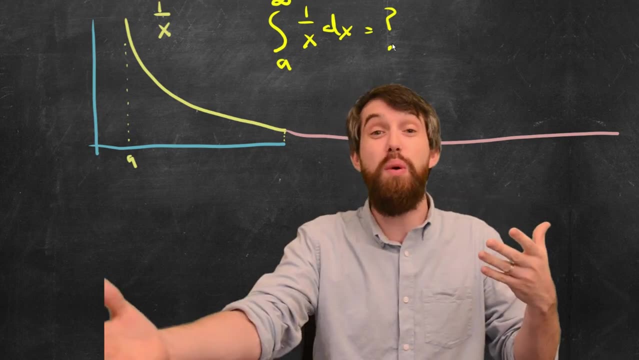 numbers. Yes, the area is going off. you're always adding more and more area, but you're adding smaller and smaller and smaller amounts each time, And sometimes that means that this area is going off to infinity, but it's actually adding up to a finite value, which is pretty. 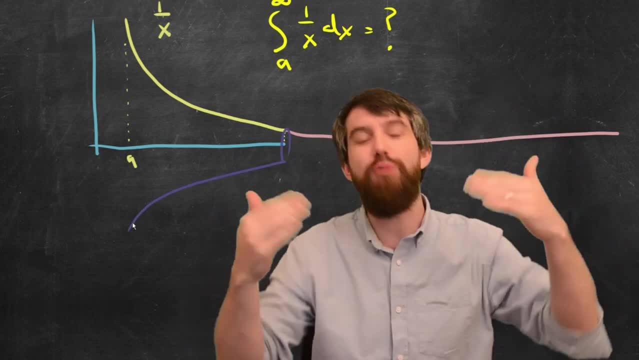 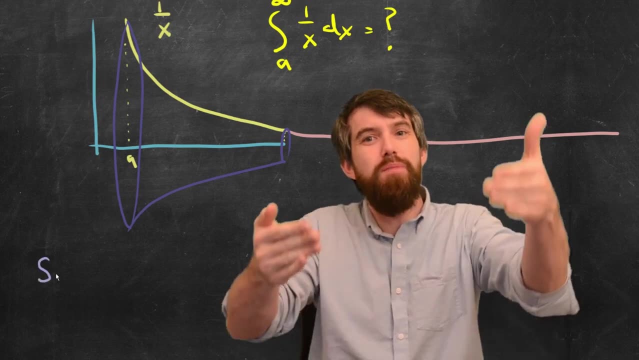 cool. Now I want you to take this curve, I want you to rotate it around the x-axis. We've seen that in Calculus 1.. However, what we can do this time is not just compute the volume, but we can compute the surface area of some region of revolution And in this particular, 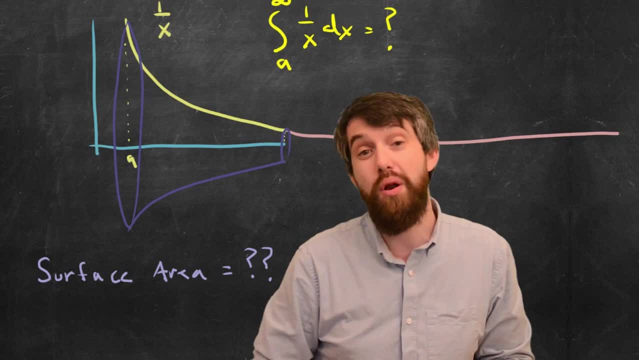 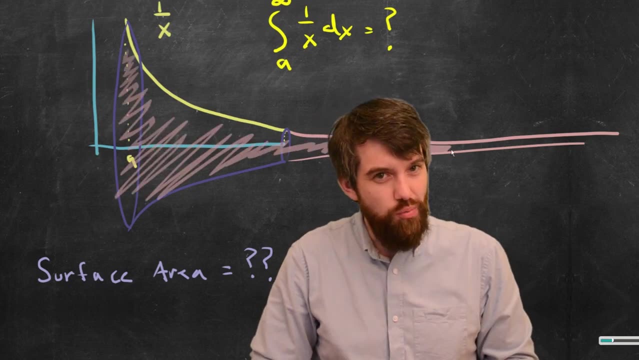 case this is something called Gabriel's Horn. in the instance of 1 over x, the surface area of this sort of infinite horn is infinite, But the volume, which we could do by our methods, from Calculus 1, the volume is going to turn. 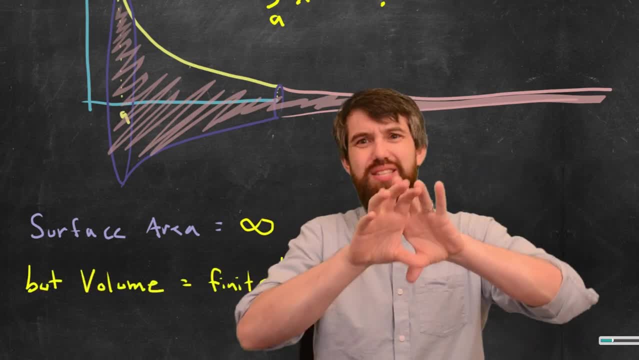 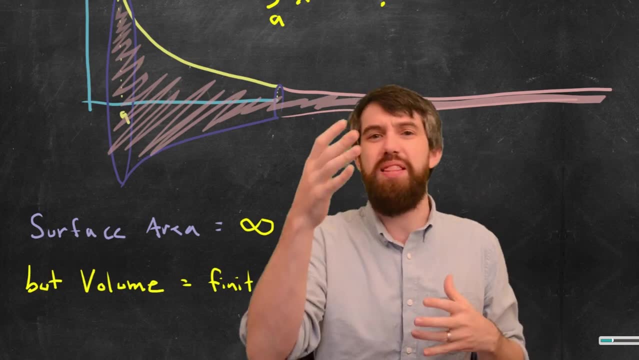 out to be finite, which is pretty cool that you have this sort of infinite region with an infinite surface area but somehow a finite volume. Along the way of developing the surface area formula, we're also going to be able to figure out how do I just compute the length. 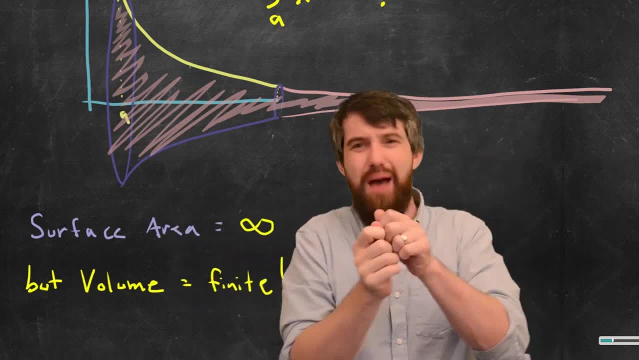 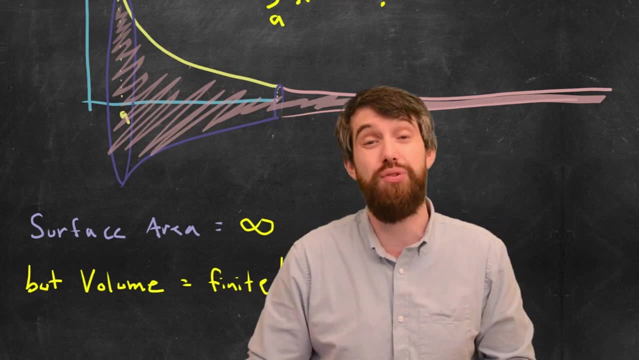 of a curve, If I just take that curve between two values. imagine I've got a piece of string and I stretch that piece of string out, This is going to be the length of that curve. this is arc length and we'll be able to answer. 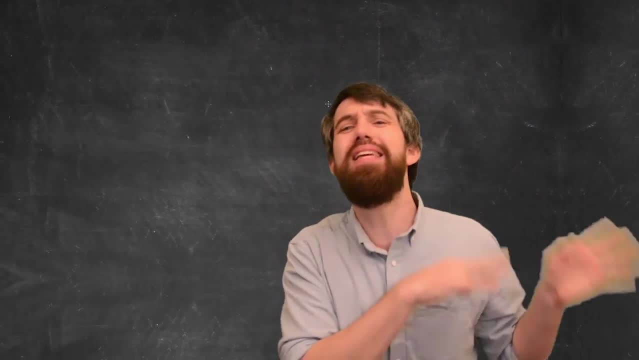 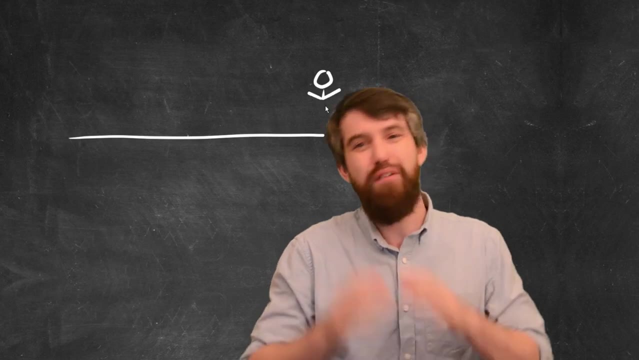 that by integration too. Now for something completely different. we're going to leave integration behind, at least a little bit. I want you to imagine that I'm trying to get out of this room. I've got here, I've got the door and I could do this in a whole bunch of steps. I can go from where. 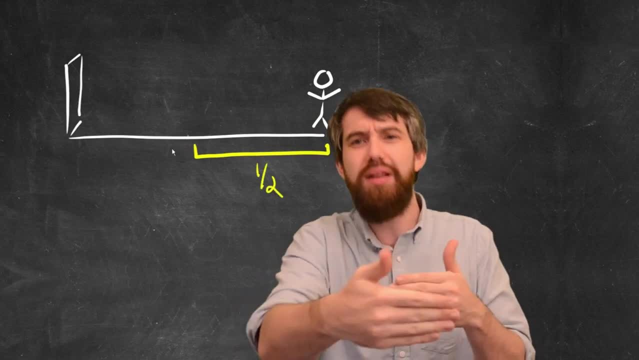 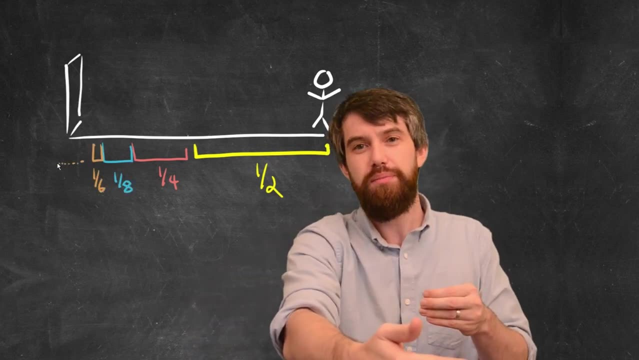 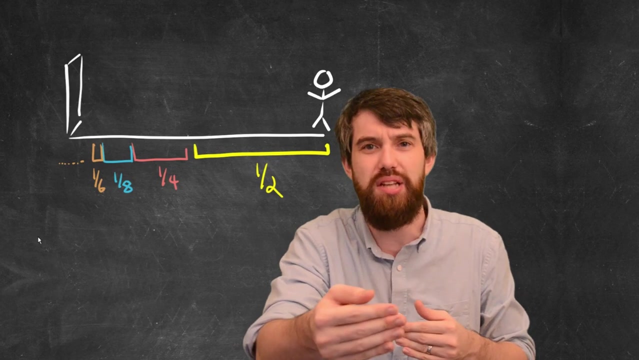 I am halfway out, And then I can go halfway out again, so half of a half is a quarter, and then I can go halfway out again, so an eighth, and then halfway out again, so a sixteenth. There's really infinitely many steps Every time I go from where I am to halfway the distance. 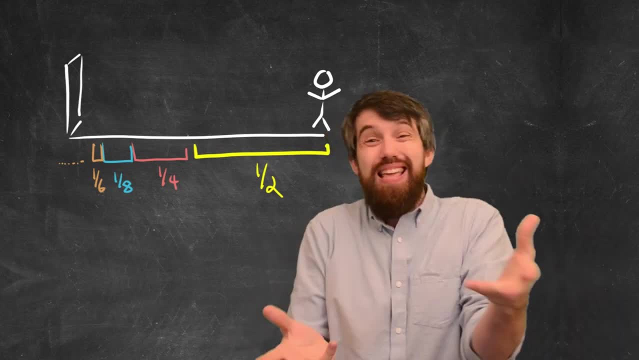 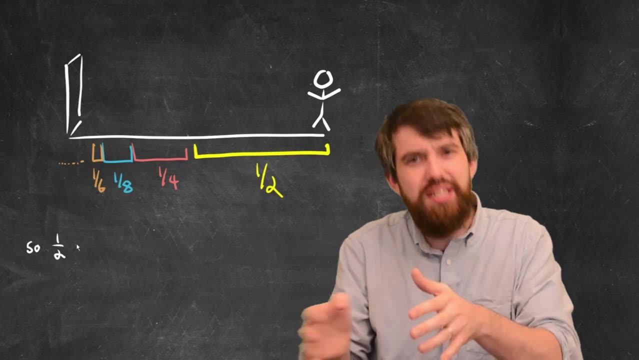 of the door and I keep on going on and on forever, But clearly I can get out of a room. So what on earth is going on here? It's the idea that the sum of a half and a quarter and an eighth, and a sixteenth, and a thirty-second, and a sixty-fourth and a 128, and you just 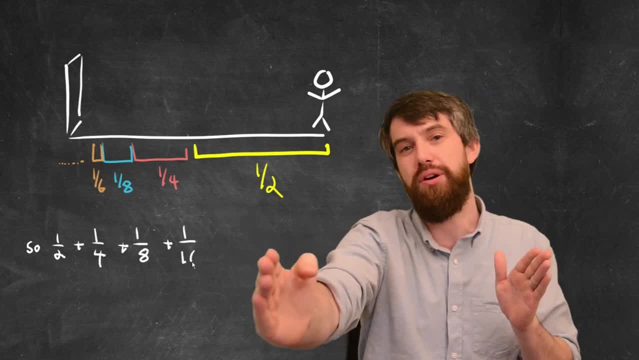 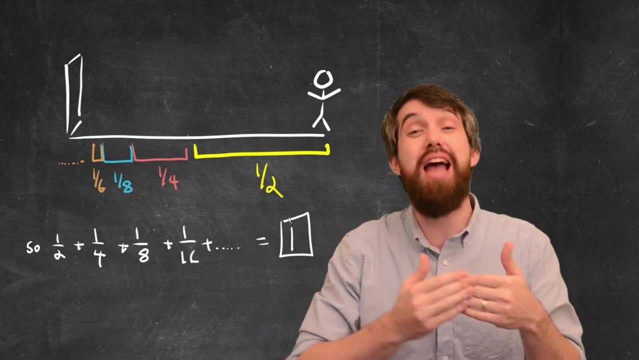 keep on going down the line that infinite sum with infinitely many terms is not infinity, It's one, It's 100% of the way up to the door, Which is a pretty cool thing that you can have these infinite sums and sometimes, like those improper integrals, sometimes they're. 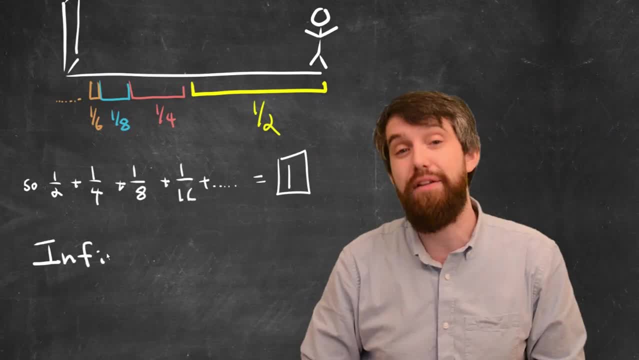 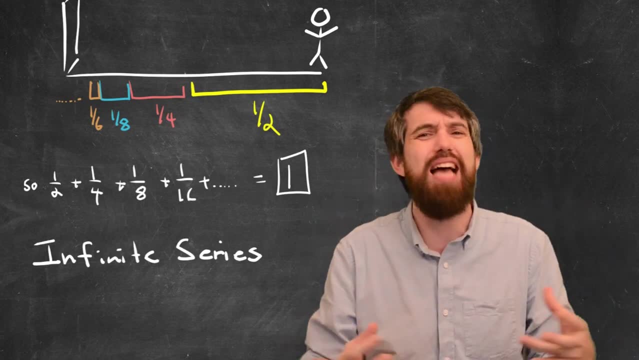 going to converge to an actual value like one. sometimes they will diverge to infinity And, if you can imagine, an infinite sum being added up and we're going to have to develop a ton of different methods to test whether it converges, whether it diverges. it's going. 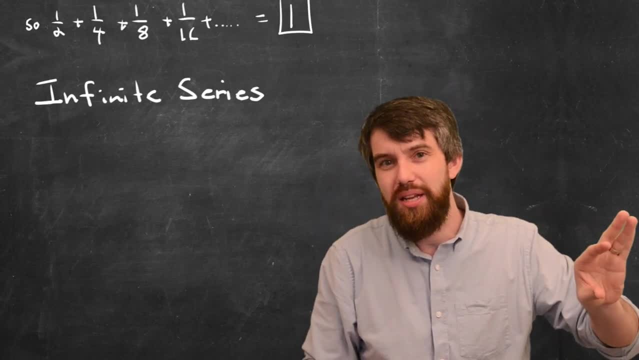 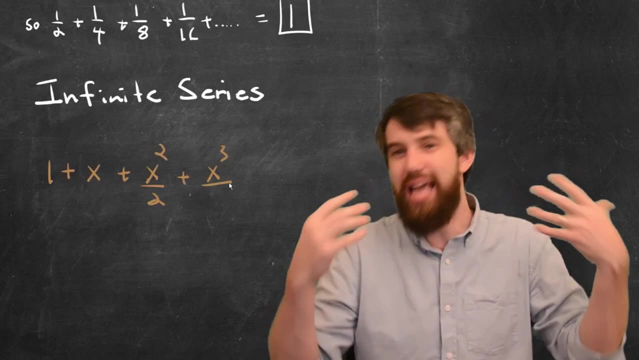 to be this whole project. But if I can imagine it for numbers, what if I added up each sum, let's just say a polynomial, a different power of x, something like 1 plus x, plus x squared over 2, plus x cubed over 2.. 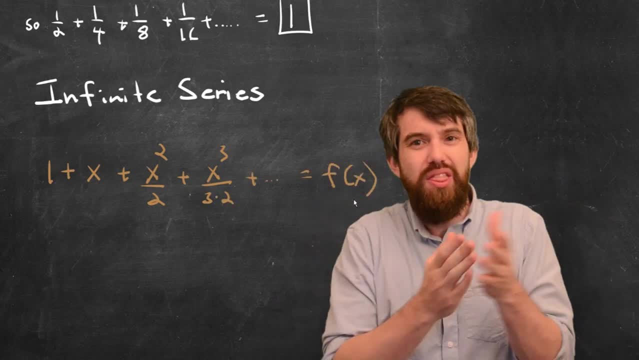 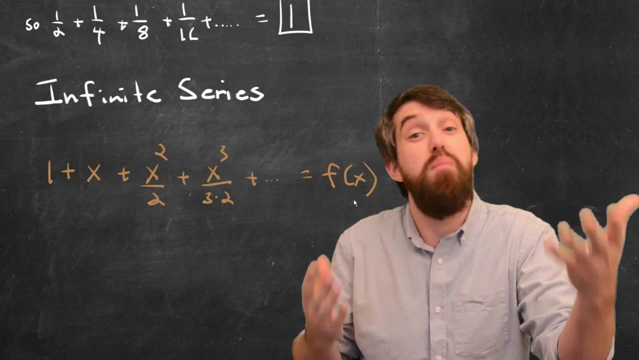 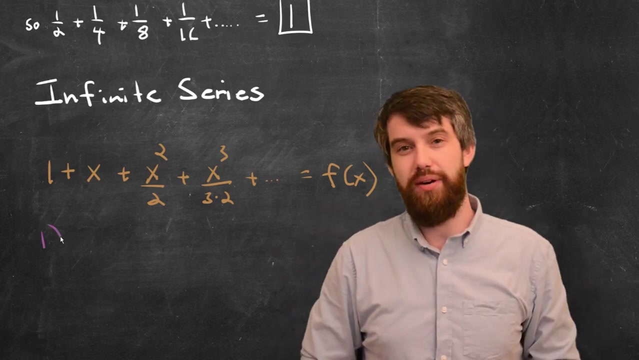 Well, this thing is some function. For every value of x, you're going to get an infinite series, and then infinite series may or may not converge And it turns out this infinite series, this 1 plus x, plus x squared over 2, and so on. this is a very special series. 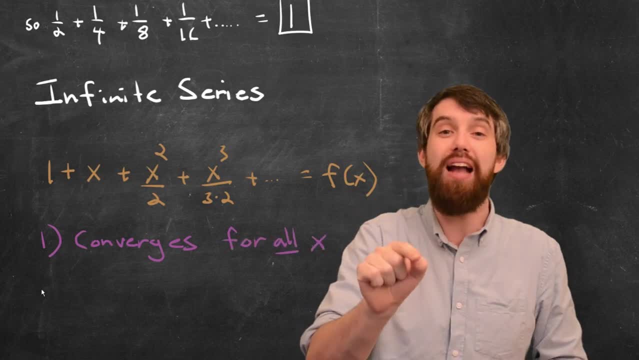 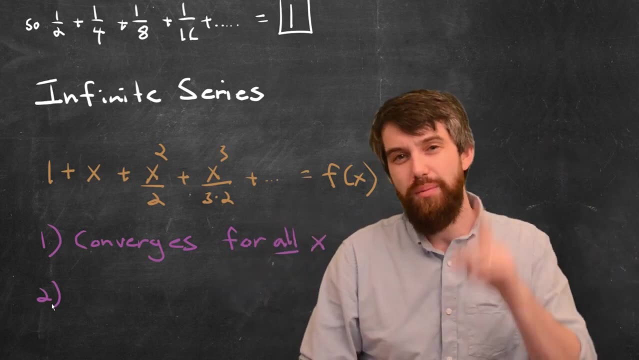 It does converge, In fact, for every possible value of x it converges. Some series only converge for some values of x, not others. This converges for every single value of x. So I'm going to capture this fact that, if you consider it more imaginatively, if you 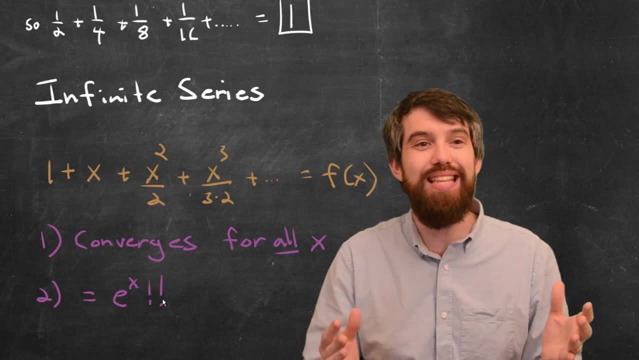 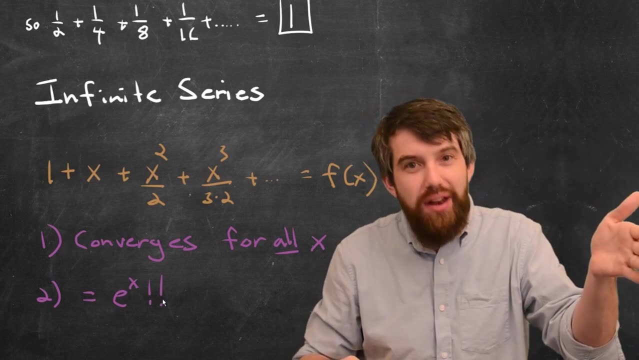 compare this to the sum. the number of set points times the sum is the same function as just e to the x. Indeed one way to see that if you take term by term and you differentiate the series, Well, the 1 goes to a zero, but then the x goes to a 1, and the x squared over 2 goes. 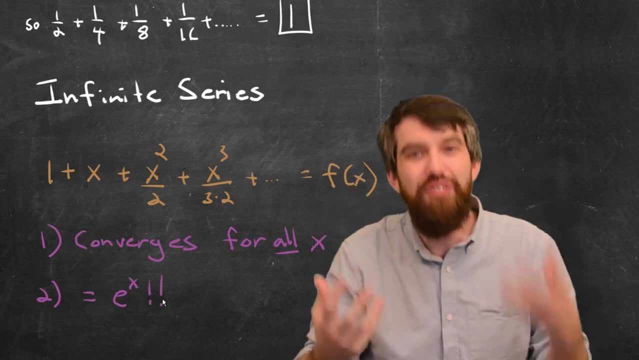 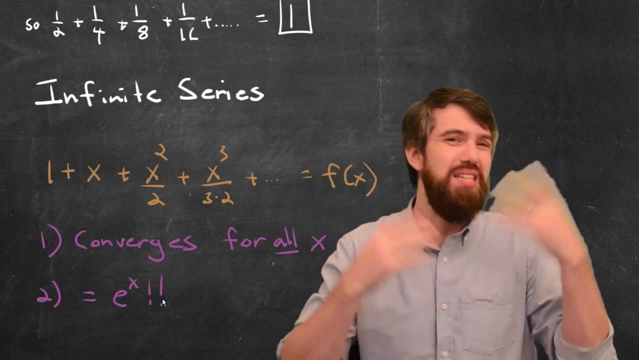 to an x Term by term. if you differentiate that series you get itself. but if you take the derivative of e to the x, you get itself as well. So that's some evidence to suggest that maybe these two things are equal and cosine and exponential. we're going to see that they all have these so-called Taylor series. 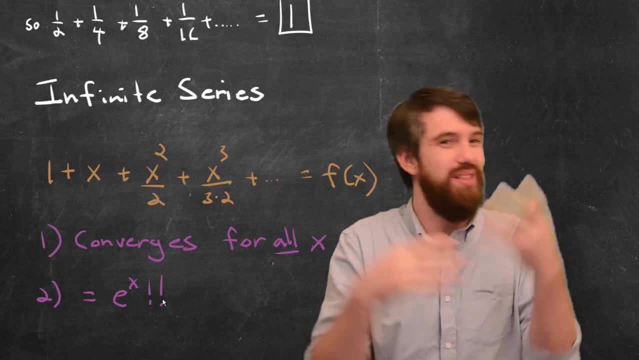 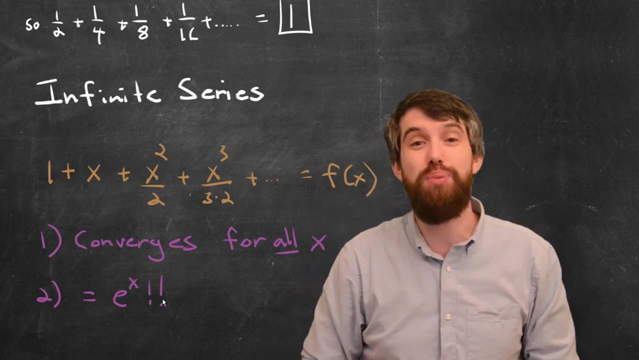 that are going to be some sort of this infinite sum of polynomials and they're going to add up to these functions And you're going to have to ask: when can be this done, Or is it only true for some values of x and not others? It's going to be a big project called Taylor series, but it's. 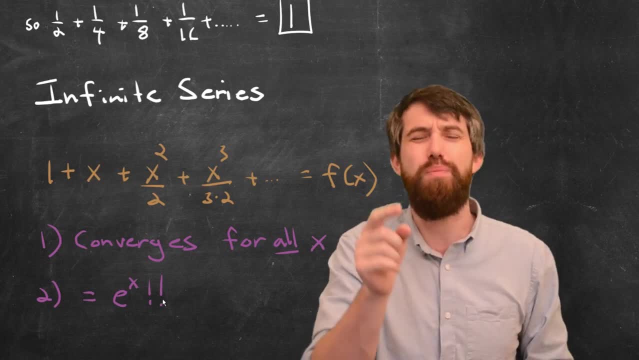 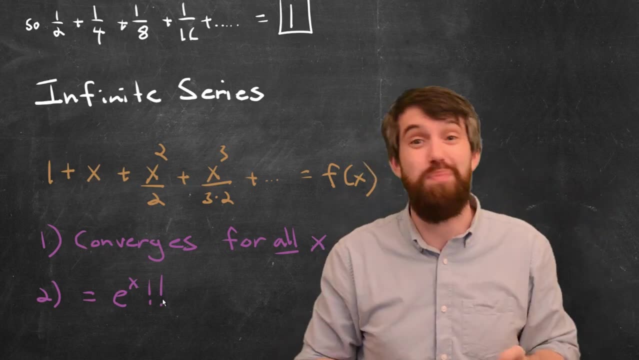 really really, really powerful, particularly because if I want to approximate e to the x, why don't I just sum up the first say three terms in its Taylor series? That's pretty simple. I could do that in the calculator. That's an approximate value for the exponential. 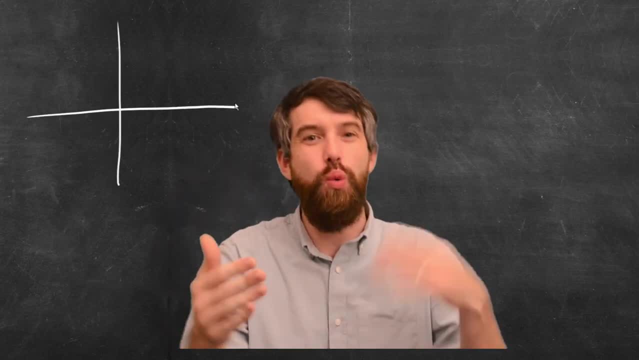 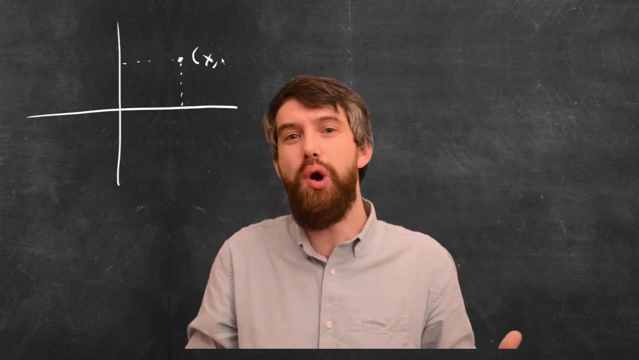 We've seen before so-called Cartesian coordinates, where I give you an x and a y, a sort of vertical and horizontal coordinate. But another, completely different way to describe points on the plane is something called polar coordinates, And here what I'm going to do is 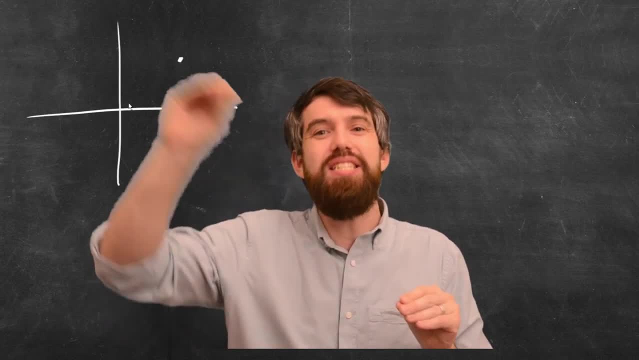 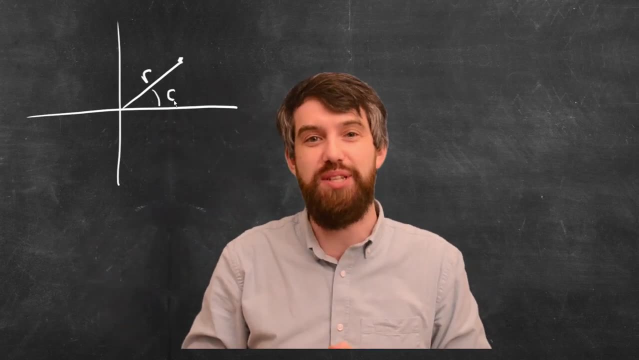 to describe some point. I'm going to tell you what the distance r is from the origin up to that point and I'm going to tell you what the angle theta from the x-axis up to that particular line is going to be. And if I give you an r, 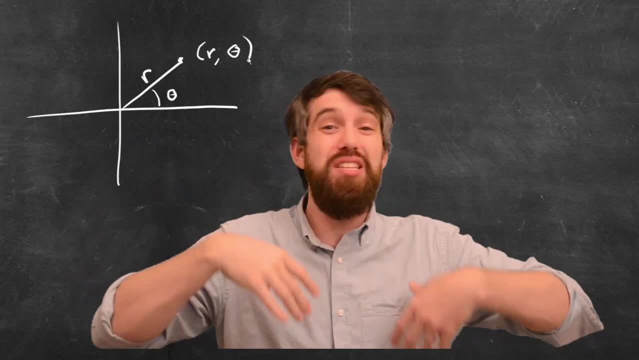 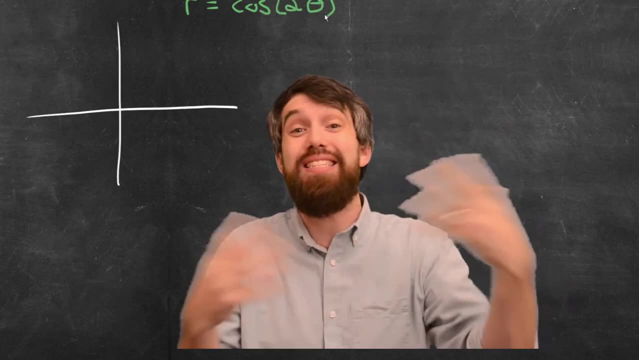 of theta, you're going to be able to plot this point. So then you're going to have these so-called polar curves. They're going to be these things like r equals cosine of 2 theta, and it's going to be some curve that exists on the plane given in polar coordinates. If I plug in theta equal to: 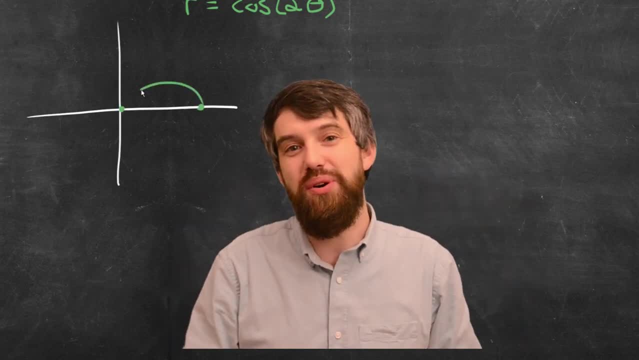 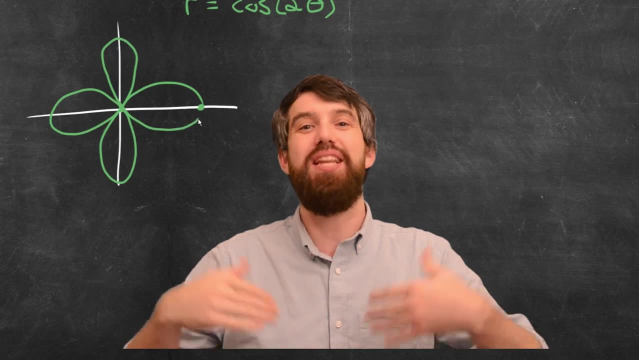 pi over 4, then my cosine is going to be equal to 0. And so if I try to plot what this point is, it's going to sort of start at 1, and then, as I rotate my theta around, it's going to get smaller. 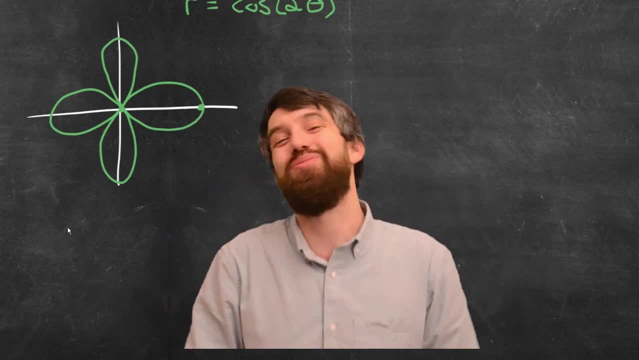 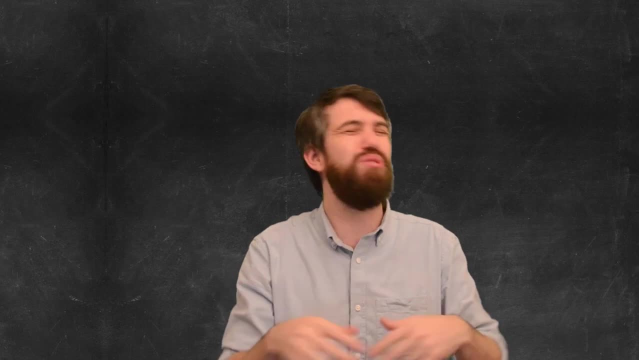 and smaller, down to 0, and then I can just continue sketching and I get this really pretty looking rose thing. So that's polar coordinates, And then the final thing we're going to look at is the idea of vectors. Now, vectors are used all the time in physics and engineering, and many of 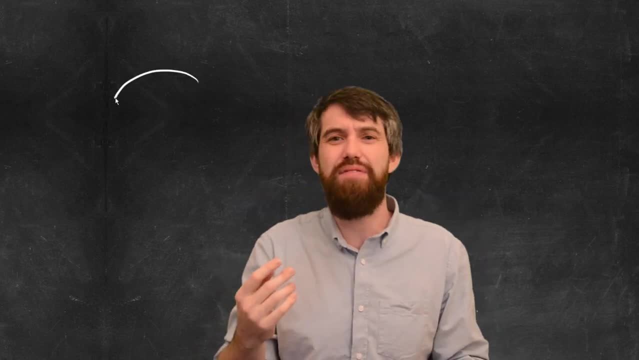 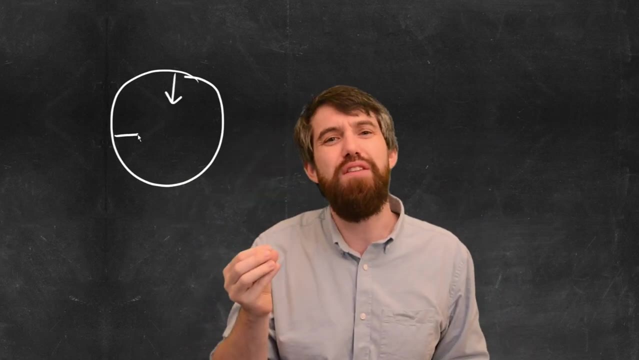 the other subjects, And one way you can think about it is gravity. If I have the Earth at every point in space, in our solar system, we have a sort of gravity force vector And what it does is it points in the direction that gravity would take me And it has sort of an 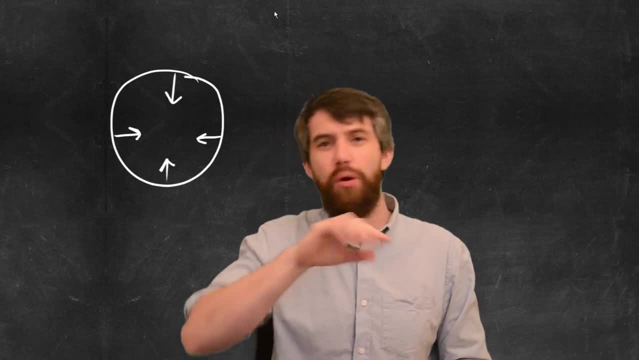 angle that's going to be the direction that gravity would take me. And it has sort of an angle that's going to be the direction that gravity would take me, And it has sort of an arrow. It tells me which direction we're going. You can see that all the way around the surface. 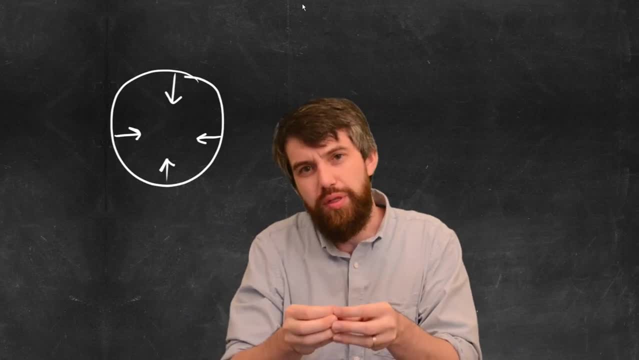 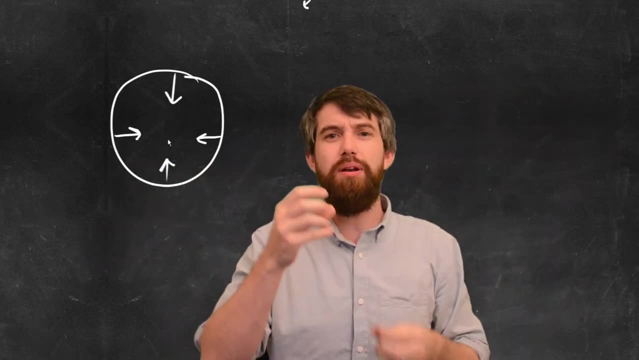 of the Earth. it's always pointing more or less to the center of the Earth. And then if I go further away, yes, it still points to the center of the Earth. I'm ignoring the sign of the moon for a little bit here, But because we're further away, the force of gravity is small, so its magnitude. 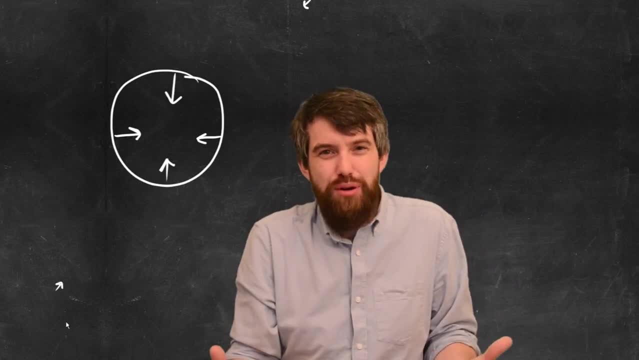 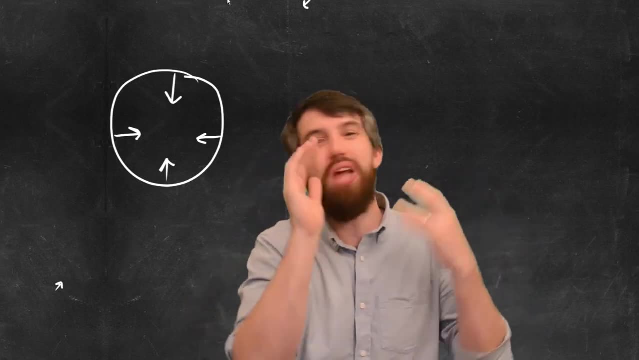 is less, And so I indicate this by the same arrow showing its direction, but the length of the arrow is a little bit shorter. So that's what vectors are. They're things with a magnitude and a direction. They're used all the time. We're going to study this in a little bit, And so 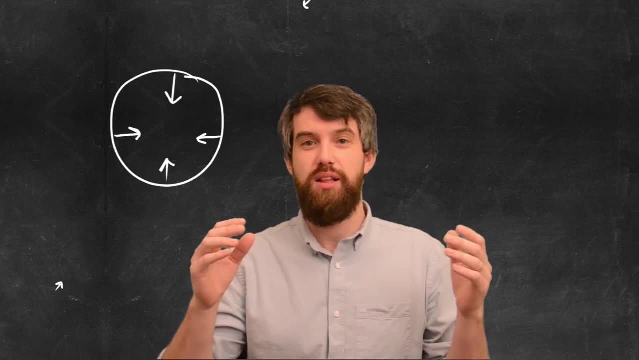 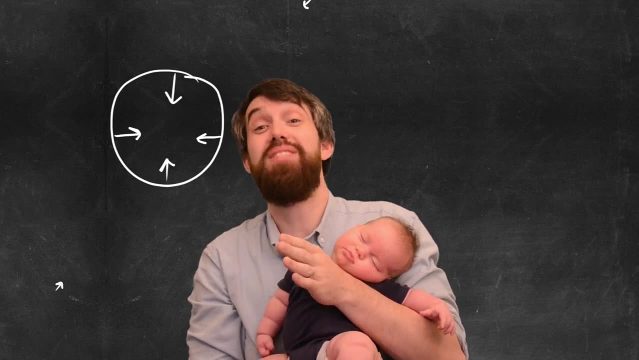 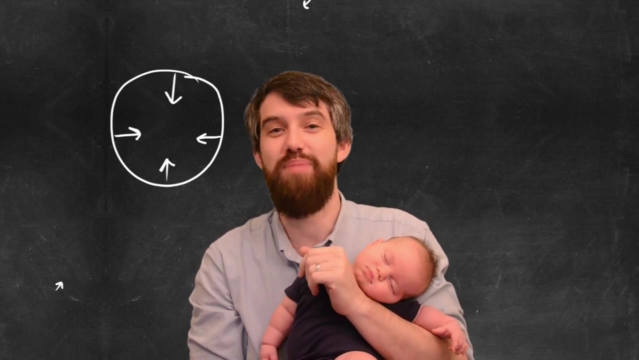 that's Calculus 2. And I know I'm excited, I know you're excited, Baby is certainly excited, And the good news here is that I already have a Calculus 2 playlist ready for you So you can go and integrate that subscribe button. Really, Integrate the subscribe button. 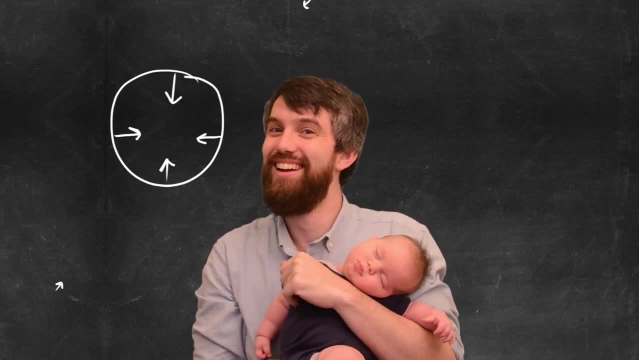 I'm trying to have my YouTube moment. Give me back my baby.